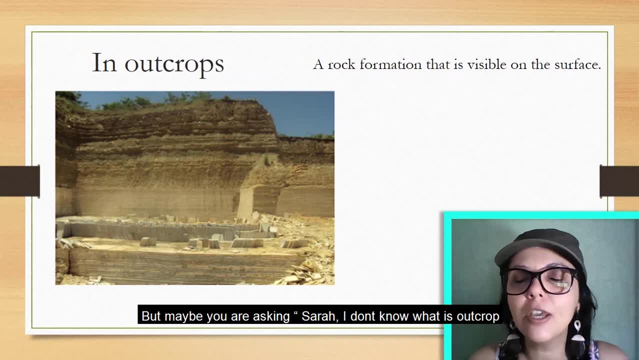 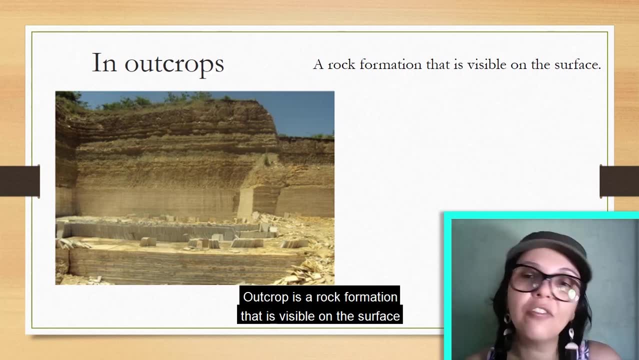 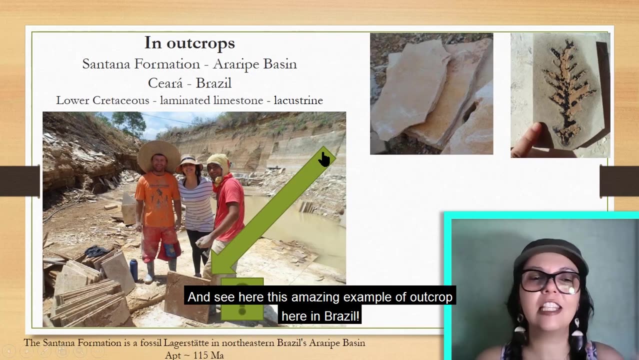 fossils in outcrops. But maybe you are asking, Salma, do you know what is outcrop? What is outcrop? Outcrop is a rock formation that is visible on the surface. See here this example, and see this amazing example of outcrop here in. 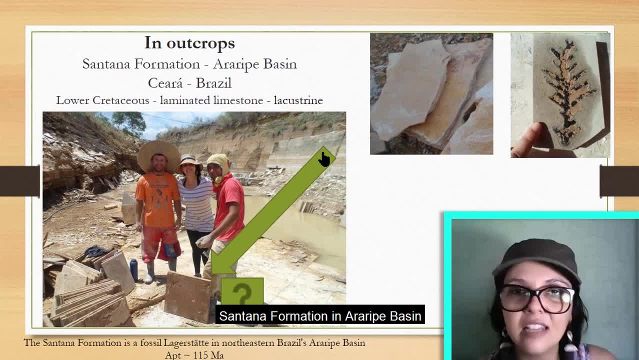 Brazil. Santana formation in Araripe Basin. this basins very important because the great outcrop is a very important part of the soil. So what is outcrop? You have to find outcrop in this area. Santana formation in Araripe Basin. this basins very important because 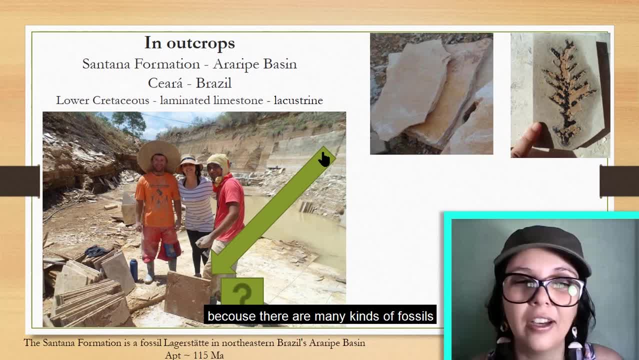 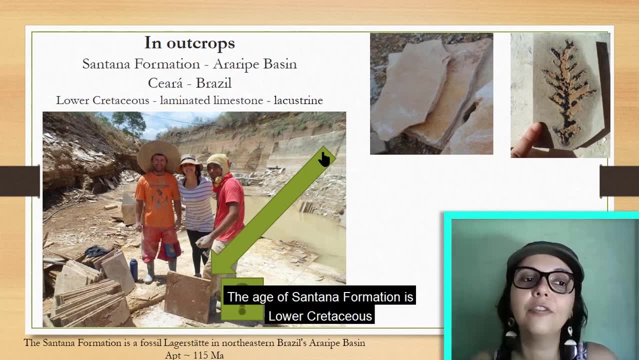 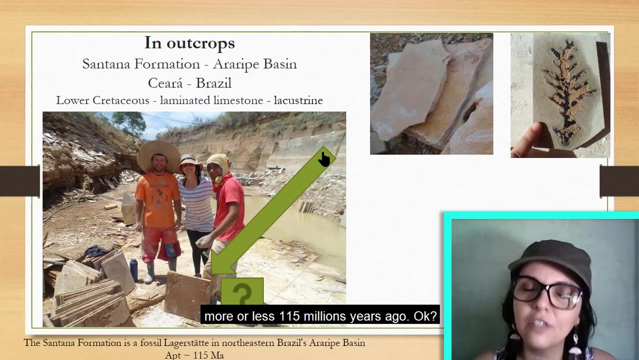 because there are many kinds of fossils. okay, Plenty of fossils, animal fossils. The age of the Santana Formation is lower Cretaceous, more specifically, Apitian, more or less 115 million years ago. okay, See here this laminated limestone. This laminated limestone was: 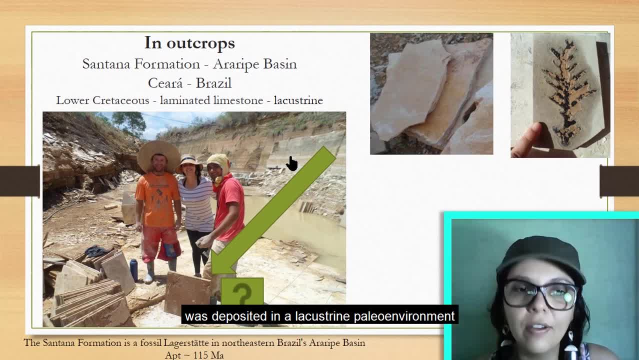 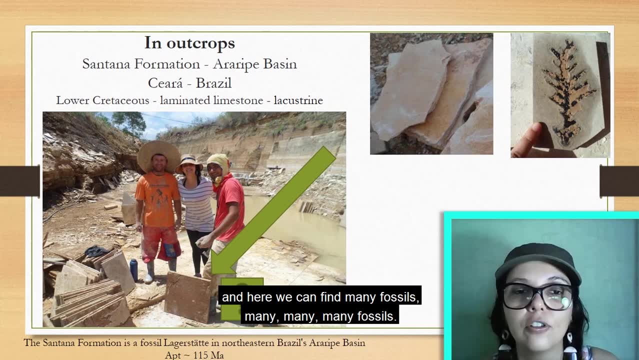 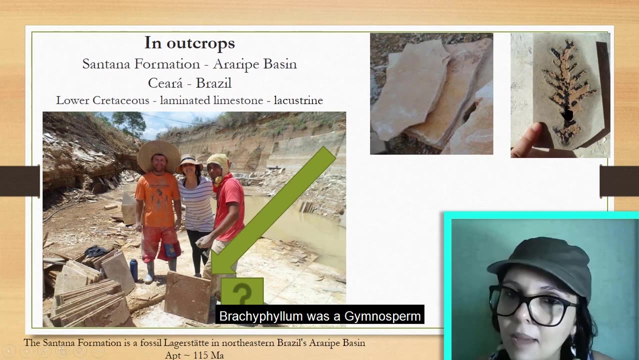 deposited in a lacustrine paleoenvironment, okay, And here we can find many fossils, many, many, many fossils. You can see here one example: Brachyphyllum. Brachyphyllum was a gymnosperm that lived millions of years ago and was preserved in this formation. 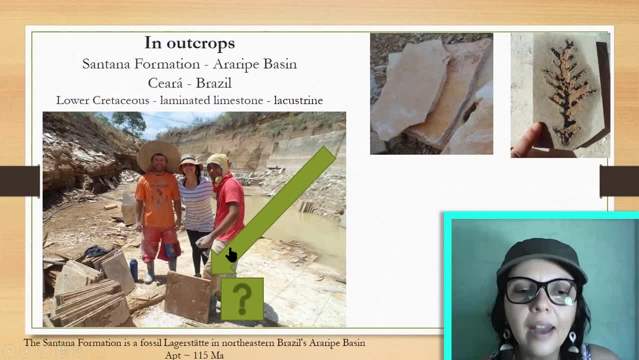 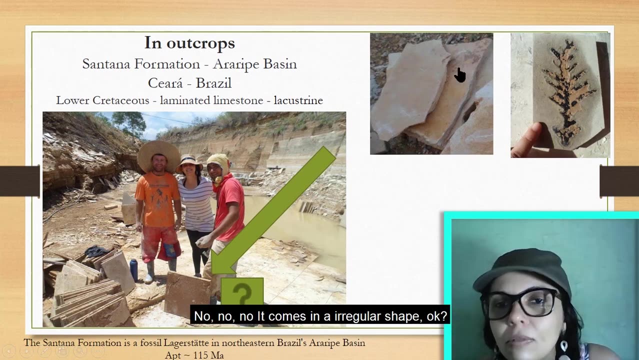 Maybe you are asking, Sara, when the paleontologists take the sample, take the rock from this formation. it comes in this way, in a regular square. No, no, no, It comes in an irregular form. okay, To put in a regular square is. 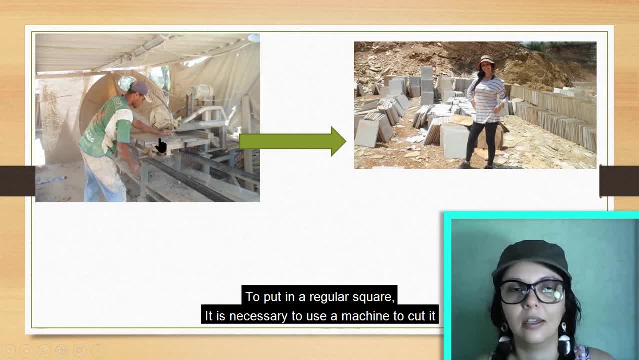 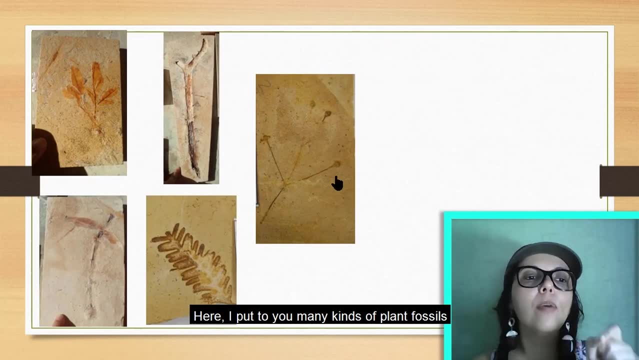 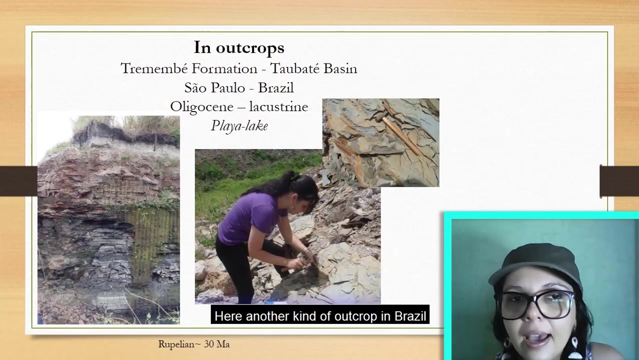 necessary to use a machine to cut it. So see here this example. Here I put to you many kinds of plant fossils found in this formation. see Very beautiful Here, another kind of aceticlop in Brazil, Trememberg Formation, Taubaté Basin in. 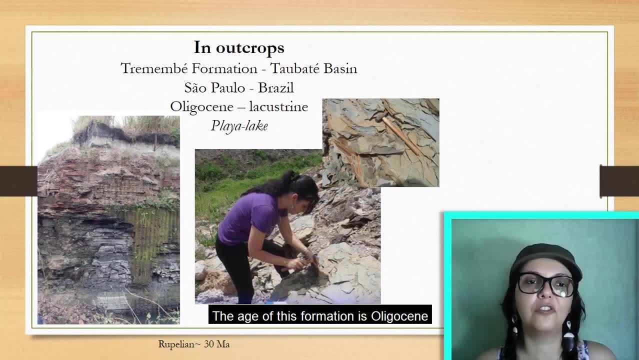 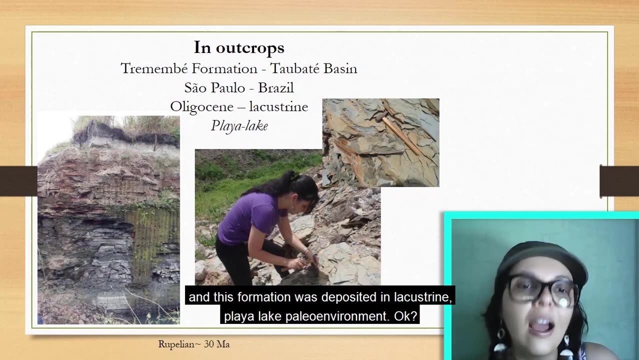 Sao Paulo state. okay, The age of this formation is Oligocene, more specific, maybe Rupelian, 30 million years old, years ago. and and this formation was deposited in a lacustrine plier lake. okay, so it's possible we find in this formation many fragments of plants preserved here. 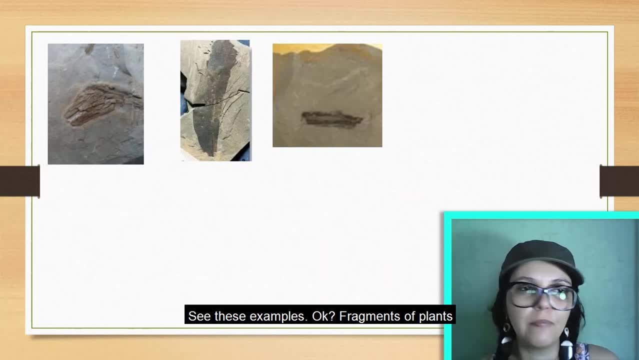 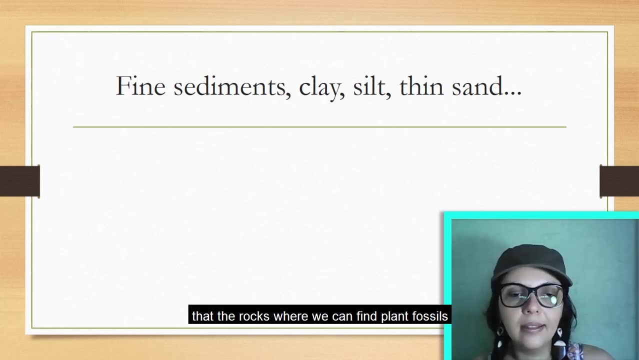 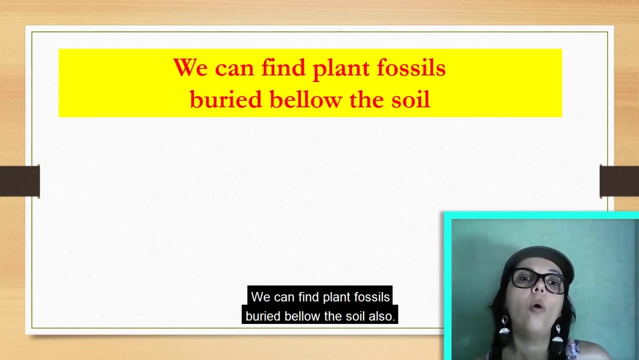 see these examples: okay, fragments of plants fossilized preserved- uh, it's very important. you know that the rocks where, uh, we can find plant fossil, in general these rocks are are with the fine sediments, for example, clay, silts, incense. okay, uh, we can find plant fossils buried below the soil also. 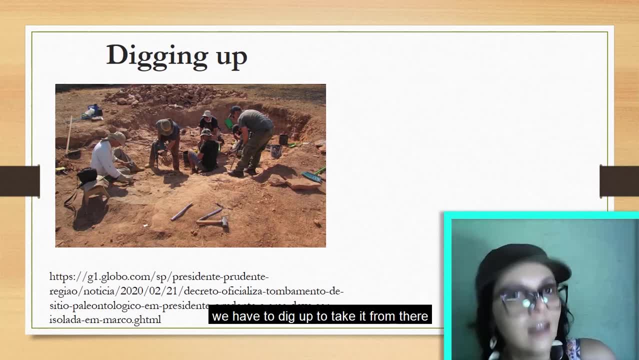 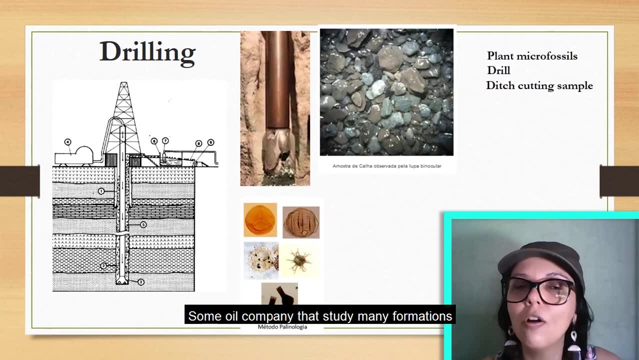 so to take it, we have to dig up, to take it from there, or drilling- okay, uh, some oil company that is studying many formations, many bases around the world in general, geologists, paleontologists, take dit, cut sample and in this kind of sample we can find plant microfossils. 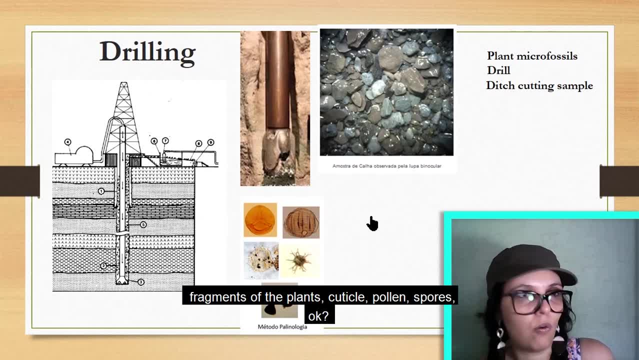 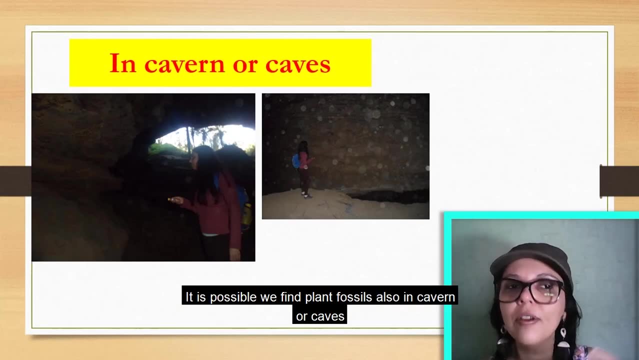 fragments of the plants, uh, cuticle, pollen spores, okay, some micro albums you can find preserved, fossilized in this kind of samples. okay, it's possible we find plant fossils also in cavern or caves. you see here in general pollen spores. so here someré. 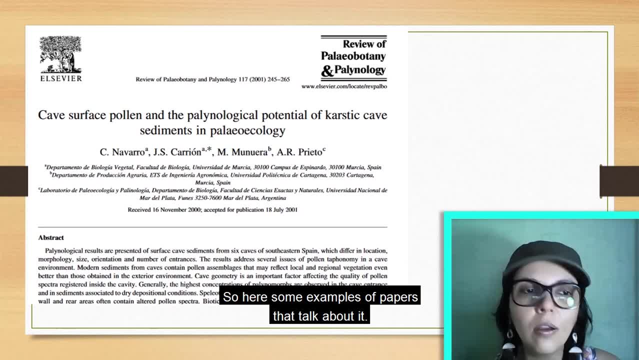 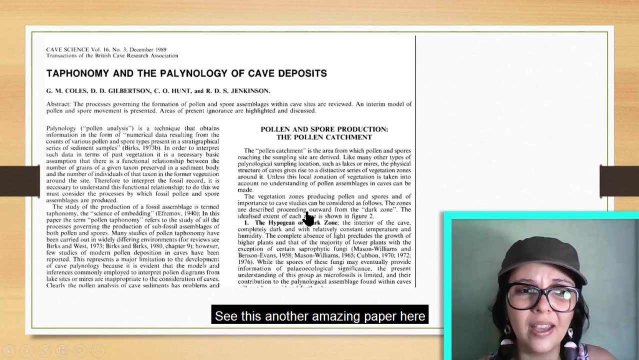 Some examples of papers that talk about it. See this amazing paper: cave surface pollen and the palynological potential of Karstic cave sediments in paleoecology. See this another amazing paper here. See it. taphonomium and palynology of cave deposits. So many microfossil plants preserved in these caves or caverns. 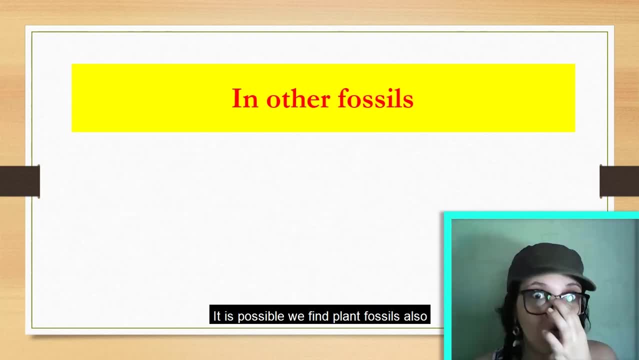 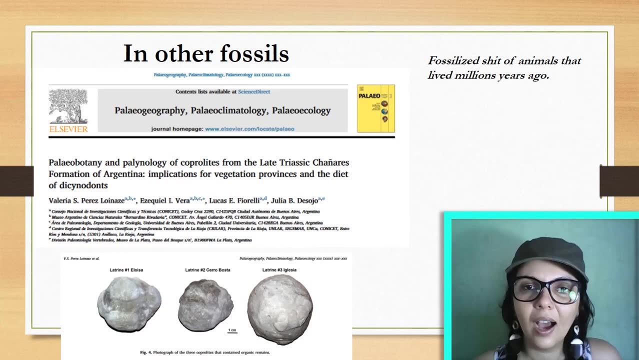 It is possible we find plant fossils also in other fossils together with other fossils, For example in coprolites, Saradonodes, coprolites, Coprolites is a fossilized sheet of animals that lived millions of years ago. So it is possible we will find in these coprolites fragments of the plants: tisus cuticulus, pollen, spores. 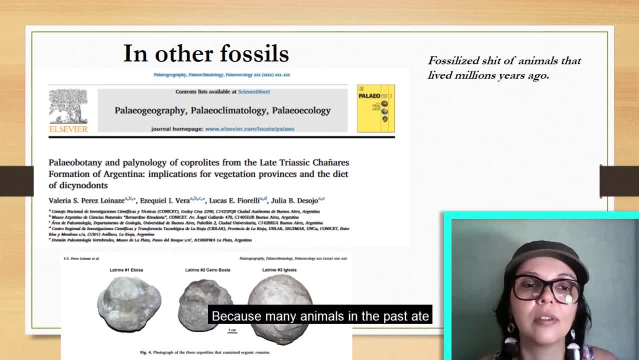 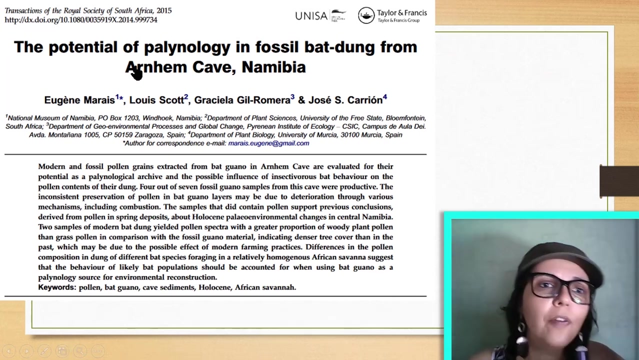 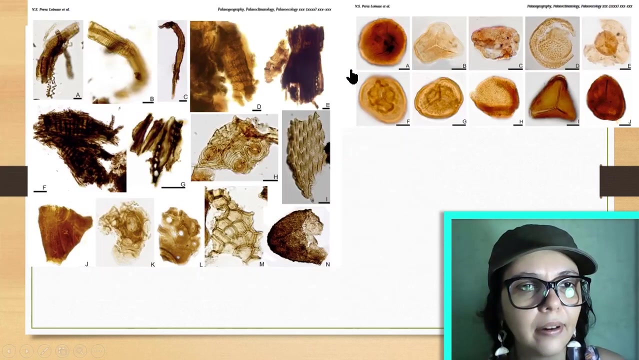 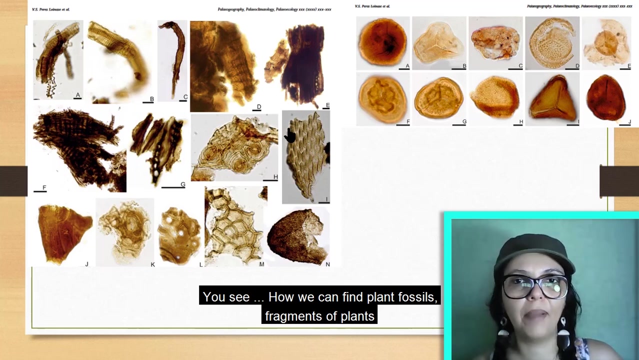 Because many animals in the past ate plants, So these fragments of plants was preserved in this kind of fossil. So you see here this another amazing paper, The potential of palynology in fossil bathodon- Very interesting paper And see how we can find plant fossils, fragments of plants, in this kind of fossil coprolites. 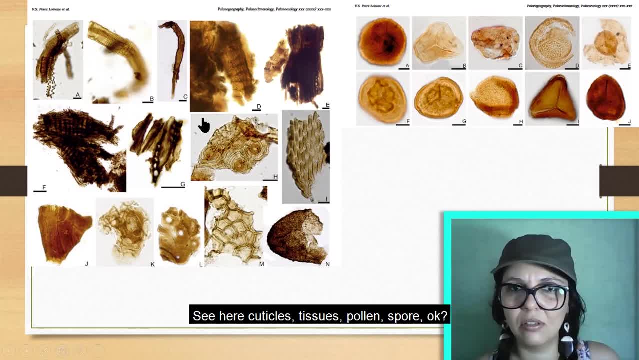 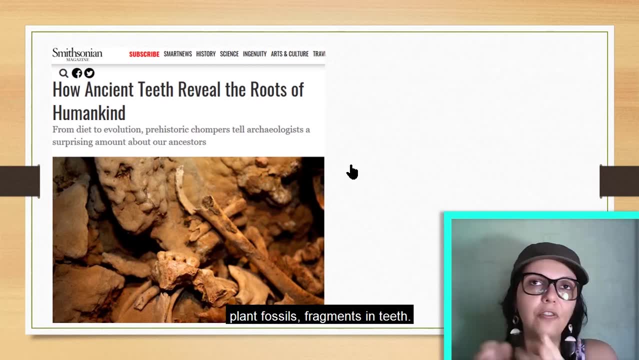 See cuticulus tisus, pollen spores. It is possible. we find also plant fossils, fragments in teeth, in preserved teeth, in fossilized teeth. It is possible, we find. So you see this amazing, this amazing paper again. 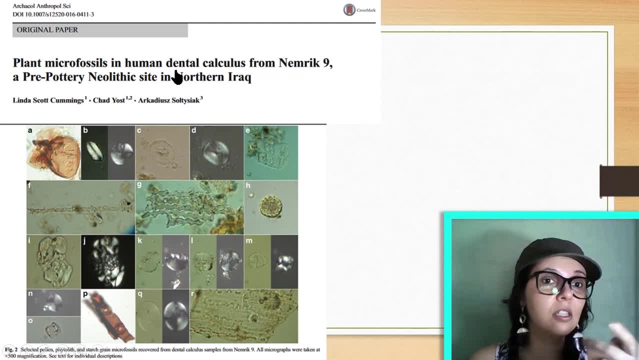 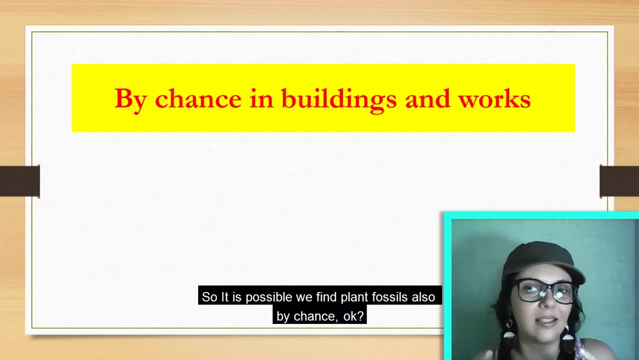 And see plant microfossil in a dental calculus. See, you can find even phytoliths, Saradonodes. watch phytoliths. So you watch paleobot video, ok, And you will learn what is phytolith. So it is possible we find plant fossils also by chance. ok. 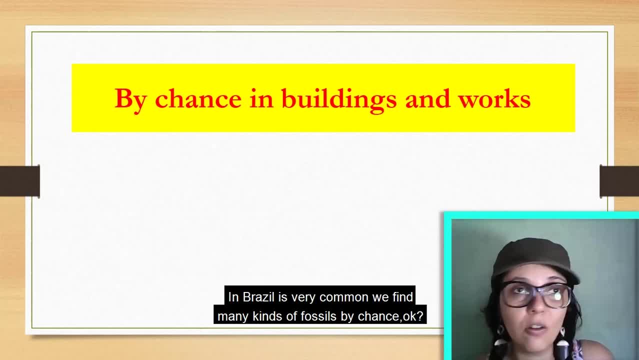 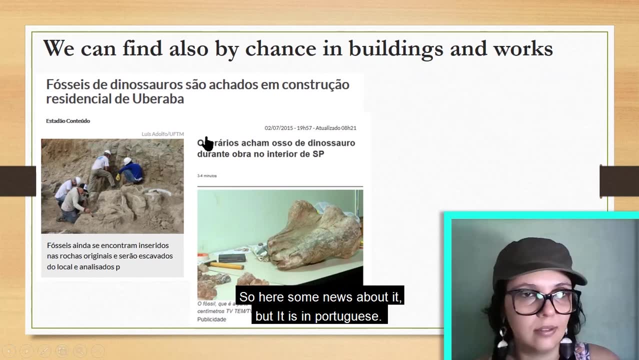 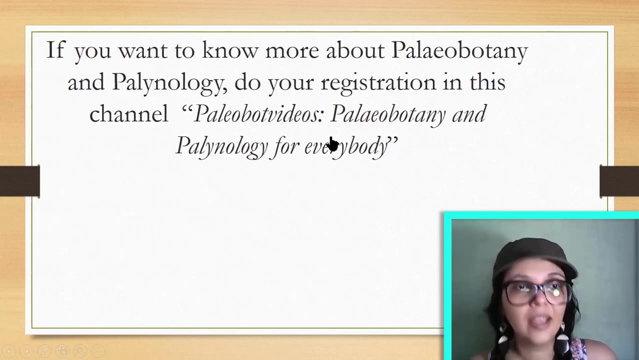 In, build and works. In Brazil it is very common. we find many kinds of fossils by chance, ok. So here some news about it, but it is in Portuguese, So if you want to know more about paleobot and palynology, do your registration here in this channel. 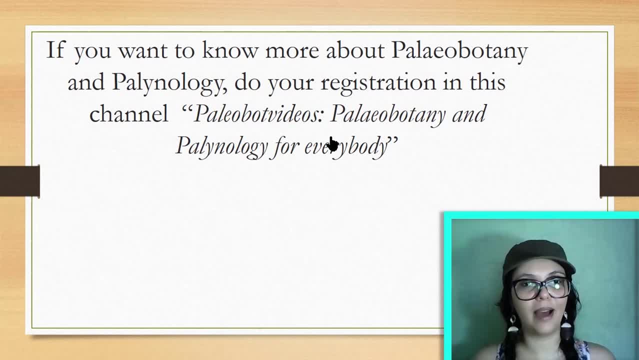 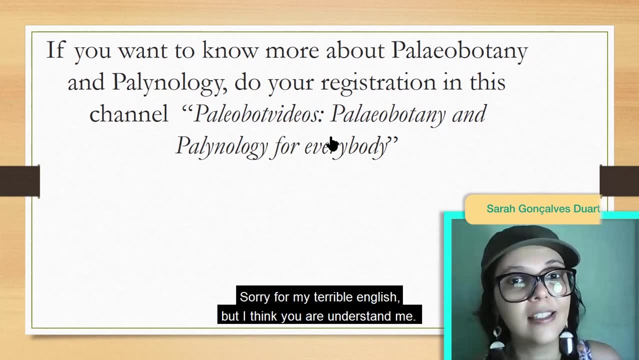 Paleobot videos. paleobot and then palynology for everybody. So thank you very much for your attention. Sorry for my terrible English, but I think you will understand me. Bye.